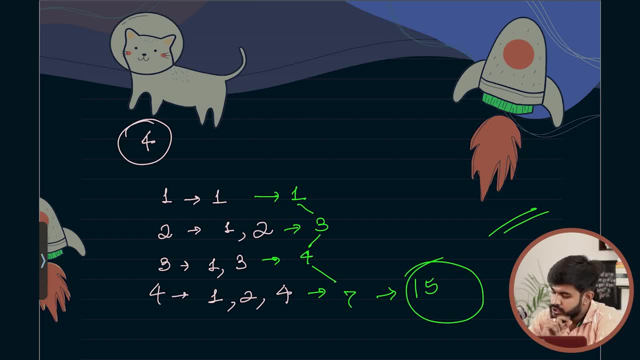 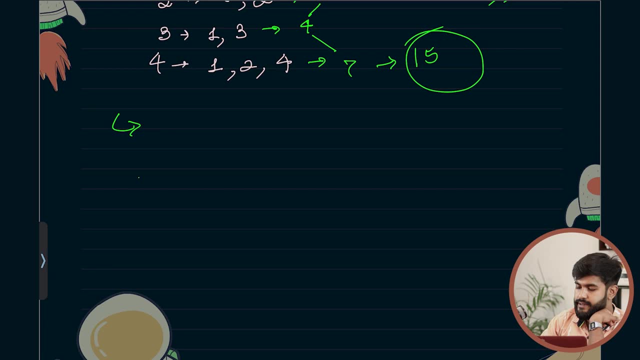 up this problem. it can be the case that you are a beginner, so i would tell you the scenario like: what is the general algorithm i have in my mind to find the divisor? the general algorithm to find the divisor of 20 is that i would start in my mind from 1. can 1 divide 20? if it can, i 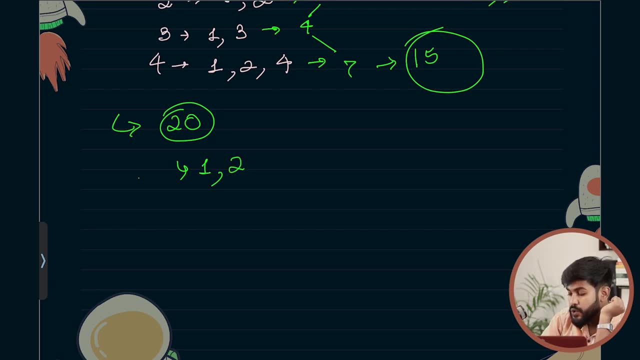 would write: 1 can 2 divide 20? if it can, i would write: 2 can 3 divide 20? no, it can't, so i would skip. 2 can 4 divide 20? yes, it can, so i would write it. so in my mind i would iterate from 1 to 20. 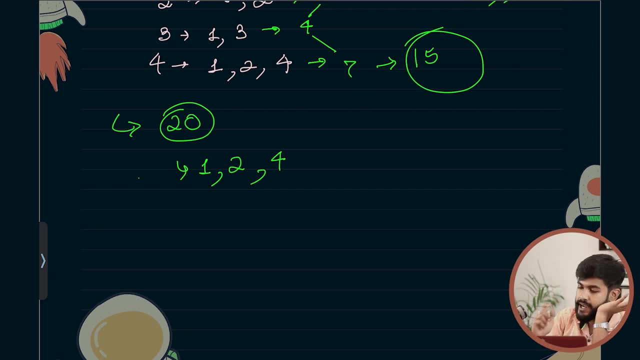 because a number greater than the number itself can't really divide it, like 21, 22 can't really divide 20. so i would go from the value 1 till the value that is given and all the values which are able to divide the number, that is, when the remainder is 0, i would say: yes, that is a divisor. so if 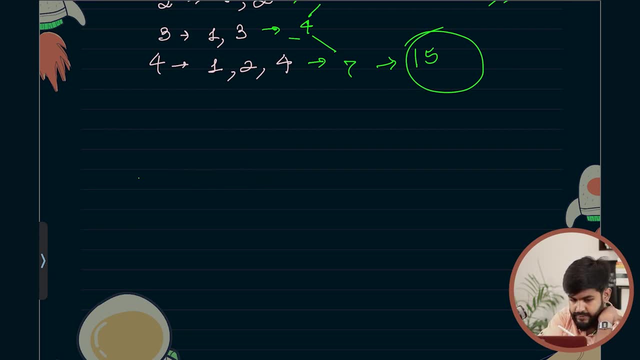 the value is, even though if this expected time complexity is not given. if the value is given n, so i would: for 1, i would go from 1 to 1. for 2, i would go from 2 to 2. for 3, i would go from 1 to 3, this would be 1 to 2. for 4, i would be going from 1 to 4 and i would be going till the value of n. so for each number, i am doing n operations. in general i can say so. for 1 number, i am doing n operations. i can say that roughly. 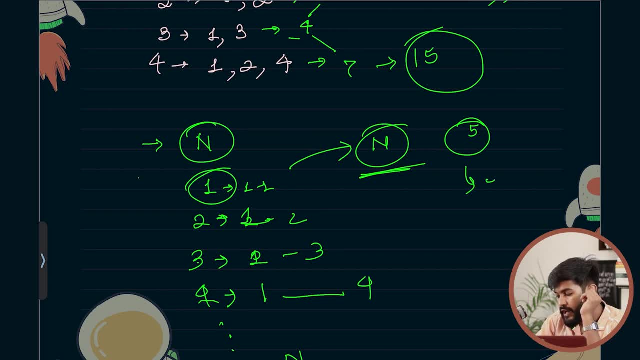 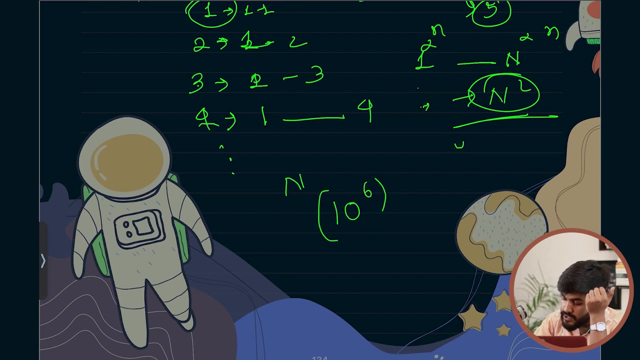 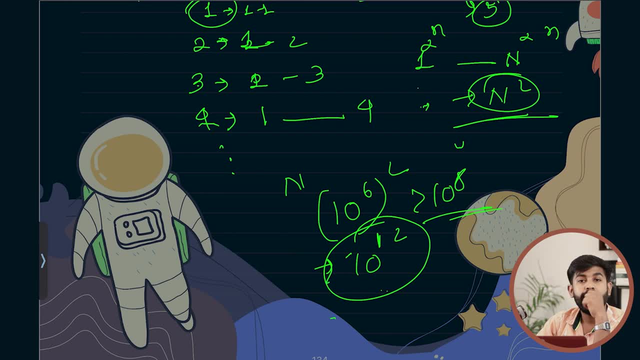 is greater than 10 to the power 8. so we would get a time limit exceeded because in one second in online compiler we can perform on 10 to the power 8 operations. so this is how i come to the conclusion that when our optimized version is needed, when it is not needed, even though this 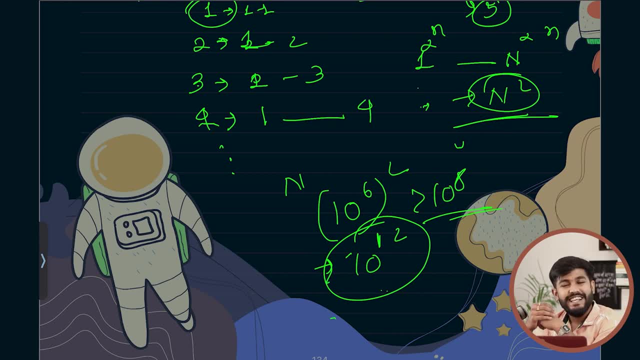 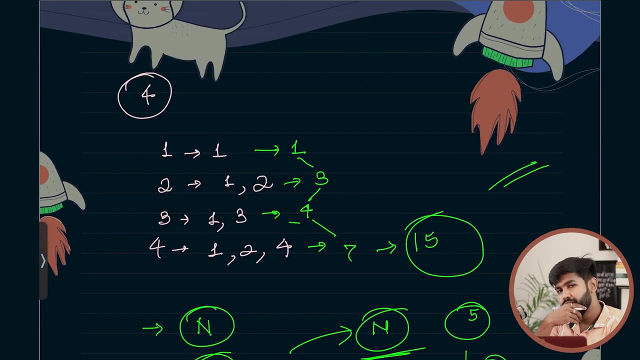 expected time complexity is given or it is not given. so this is how we get the expected time complexity. okay, so let's move forward to this. so let's just see what was here at this point, like we really want the sum so we can use a contribution technique. okay, like this is: 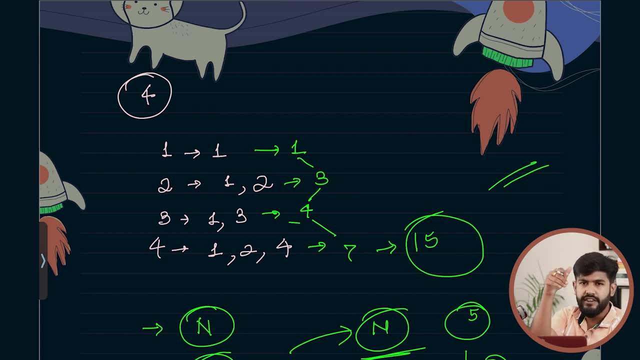 technique is known as contribution technique. if you are kind of very drilled inside competitive programming then you would know. else this is a very simple thing, like you would see. what is the contribution of each of the number in the answer? because we don't really need the values individually, like we don't really need the divisors individually. 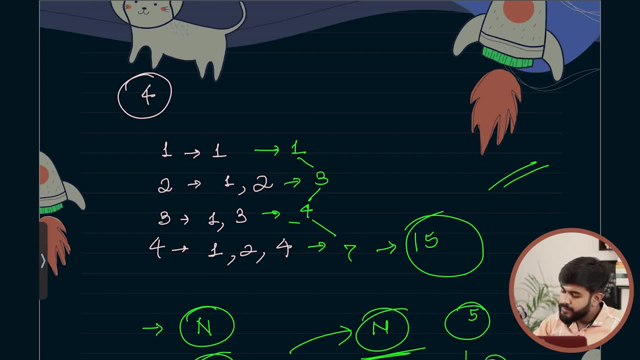 we just need the contribution as a sum. so now let us see. 1 can contribute to which all as a divisor? 1 can contribute to everyone as a divisor. who can contribute to all the events numbers in the divisor? 3 can contribute to 3, 6, 9, 12. so now let us see. 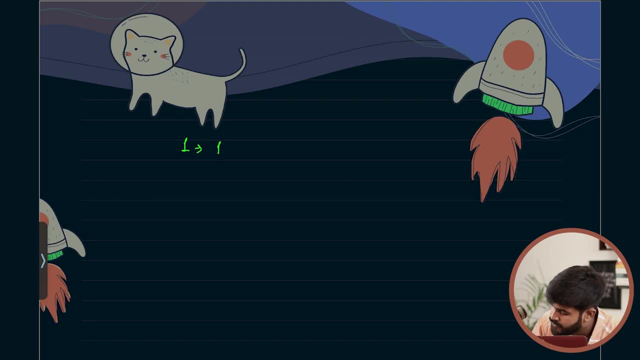 for more than value. So for 1,, the value would be 1.. So for 2,, the value would be 1 and 2.. For 3,, the value would be 1 and 3.. So for 4,, the value would be 1,, 2, and 4.. So for 5,. 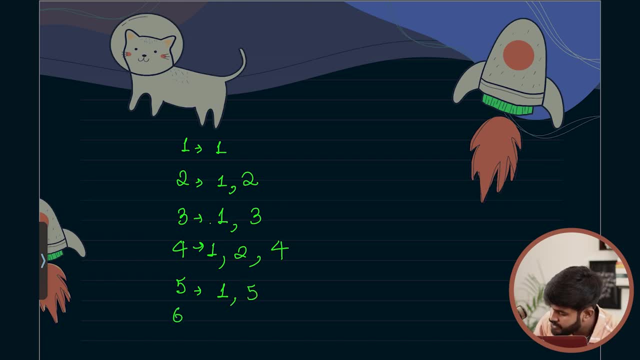 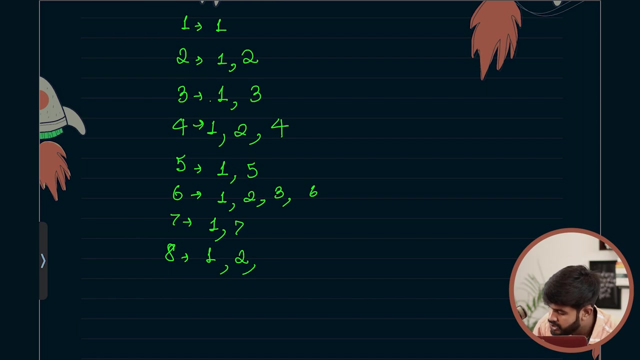 the value should be 1 and 5.. So for 6, the value should be 1,, 2,, 3 and 6.. For 7, the value would be 1 and 7.. For 8, the value would be 1,, 2,, 3,, 4, and we can't really move forward Now. 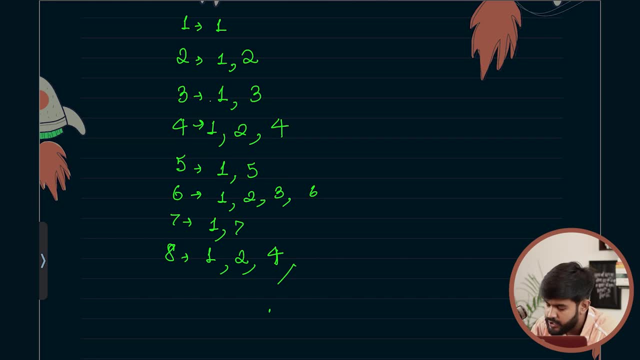 it is sufficient enough. So now we want the contribution. So we would be marking up all the numbers that we are getting, So 1 would be contributing in everyone. So if the given value is 8, so we would simply say 8 divided by 1, multiplied by 1 and the sum contributed by 1. 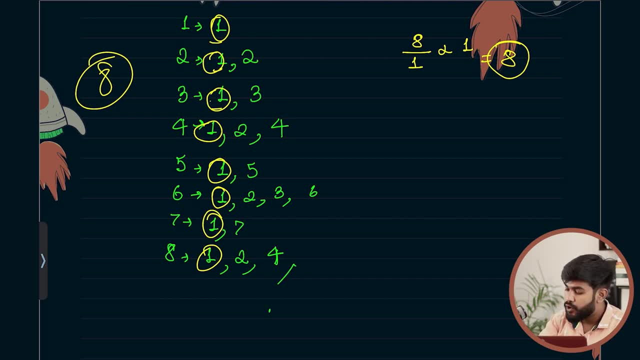 as a divisor would be 8.. Yes, it is true For 2, we have 2,, 2 here and 2 here and 2 here. So 2 would contribute to how many values? To all the even values. So 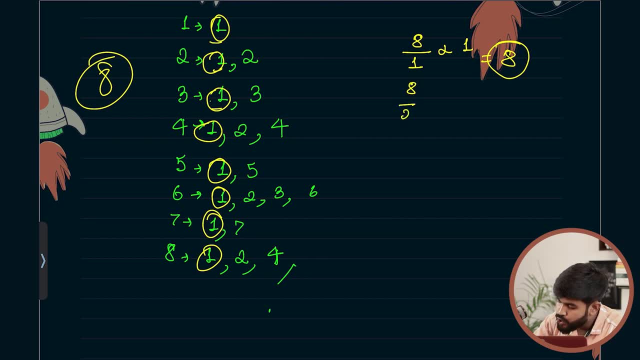 we can say that 8 divided by 2 would tell me the number of times 2 would be present as a divisor, and then just multiply it by 2, because the contribution is 2 of each one. So that would be nothing but 2, 2, that would be 8 again, and, yes, 2 to 4,. 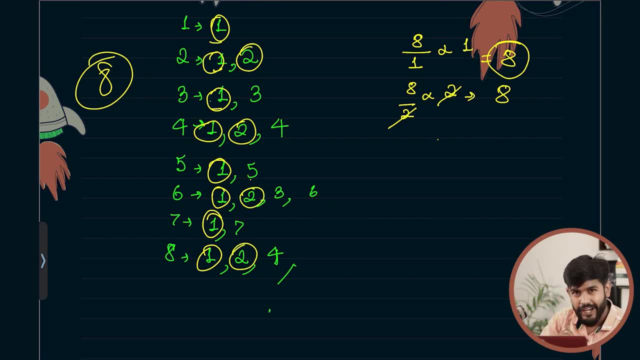 4 plus 2,, 6,, 6 plus 2, 8.. So now you are getting the idea. Now 3 as a divisor, So 8 divided by 3 multiplied by 3.. 8 divided by 3 is 2 point something, but we would take the integer value. 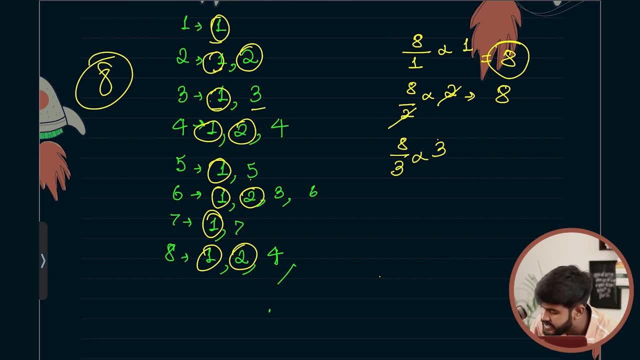 Why? Because, if you just see, 8 would be present at 3,, 8 would be present at 6.. So we are just taking that. So that would be 2 multiplied by 3. that is equals to 6.. So, yes, 3 plus 3, 6.. So 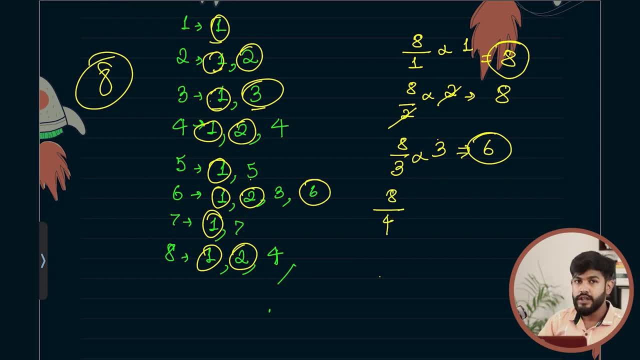 this is how we would move forward to something known as 4 also. So that would, multiplied by 4, that would be 2, multiplied by 4, that is 8 and yes, 4 is present- 2 times. Then we would be going. 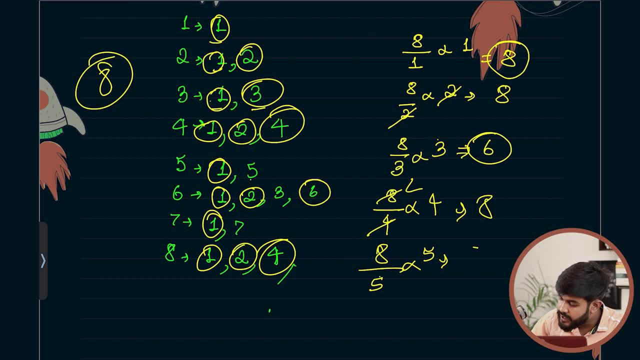 to 8 by 5 multiplied by 5, that is again 5, because 5 is present once, Then 6, then 7 and then 8 itself. Here 8 would also be present. So what we can really do is if we just add up all these values. 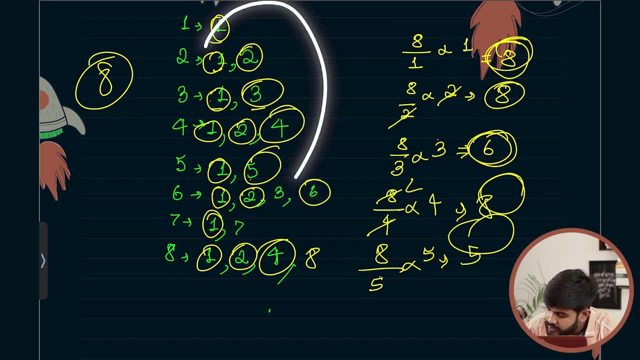 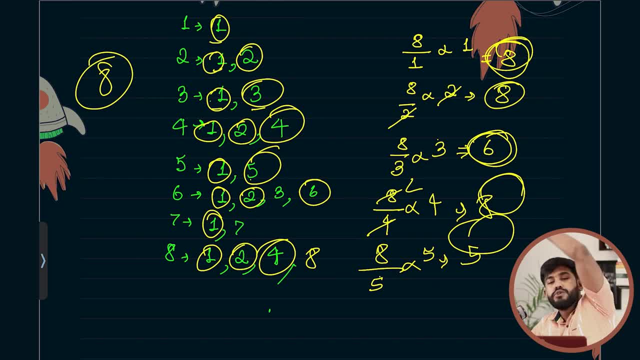 getting the individual values. we found out the contribution. Okay, like we really, really want the number of contribution multiplied by the divisor. We want this. This is what we are doing. So you just need to narrow down your thinking. If we just see the sample test case: 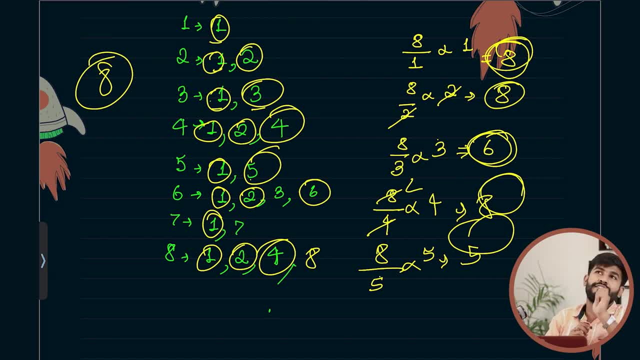 you would kind of think, okay, I need to individually find all the divisor for all the numbers, But you don't really need to do the hard work. You can just see: okay, 1 is coming 8 times, I would take it. If 2 is coming n by 2 number of times, I would take it. 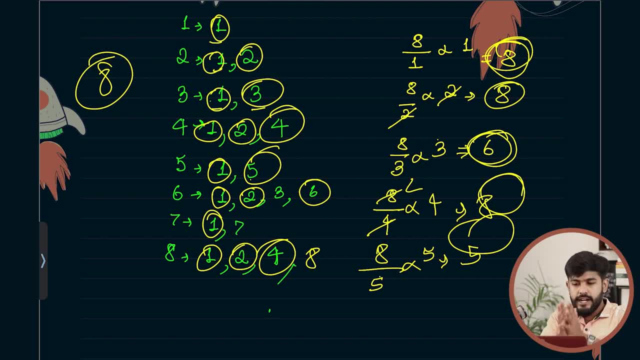 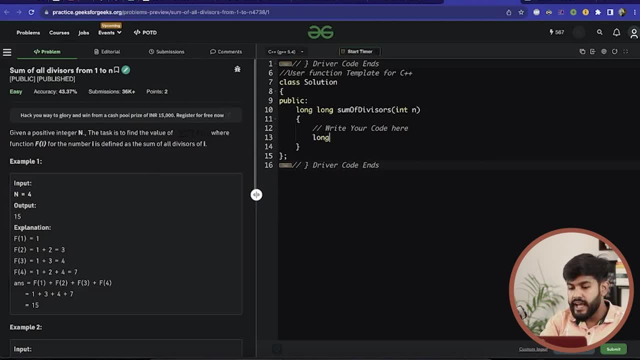 Same goes for all the individual numbers. This is how you would do it. Let us move to the implementation, and that would solve the purpose. Here we would have the value as n. So now the answer is expecting a long long. So we know the sum would be huge. So we are saving that in. 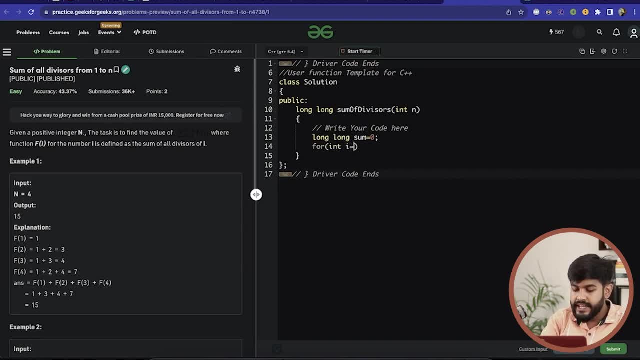 long, long. Now we would start iterating from 1.. For int i is equals to 1, we would go till the value of n and we would do i++ At each point. what we would do is sum plus equals to the total value n divided by i and 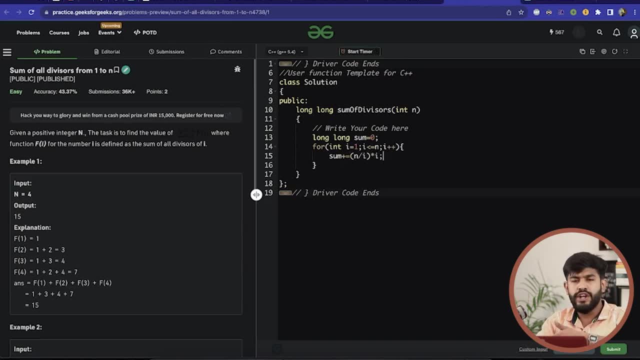 then multiply it with the value i. So this is already an integer division, Integer division multiplied by i. So we don't really like. 8 divided by 3 was 2.66, but it is already an integer division. So we would get a 2 and we would multiply it, add it, return the result. 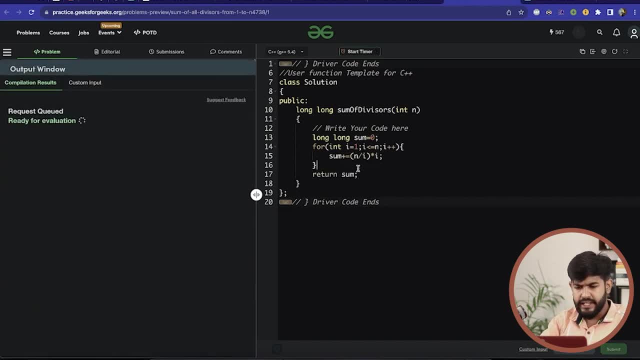 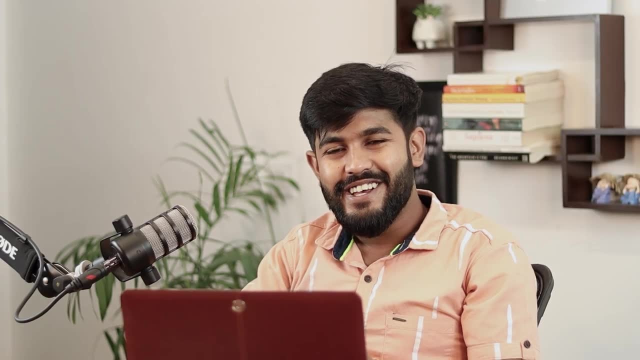 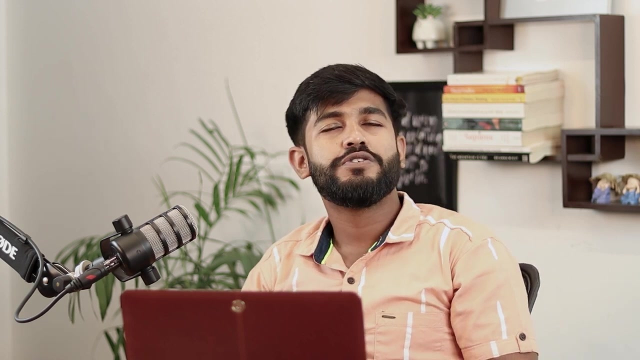 and that is sufficient. So now the time complexity is big of n. That's it. So I don't think much talking about time complexity and space complexity is needed. Only variables are used. So space complexity is big of 1 and time complexity is big of n.